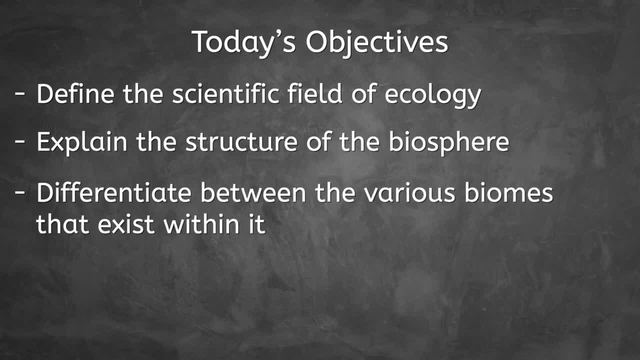 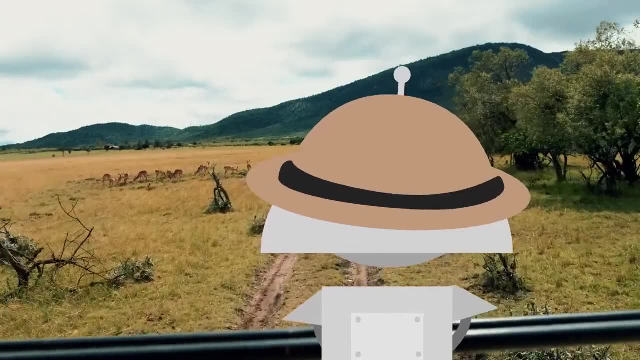 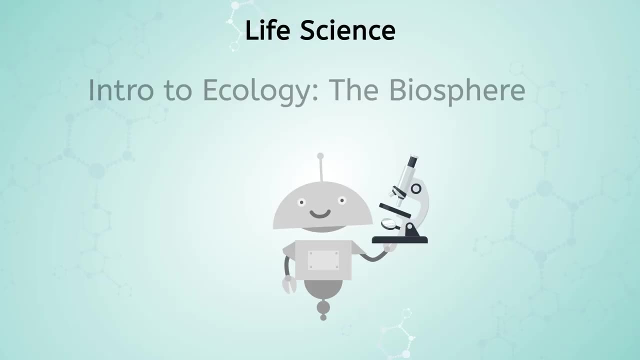 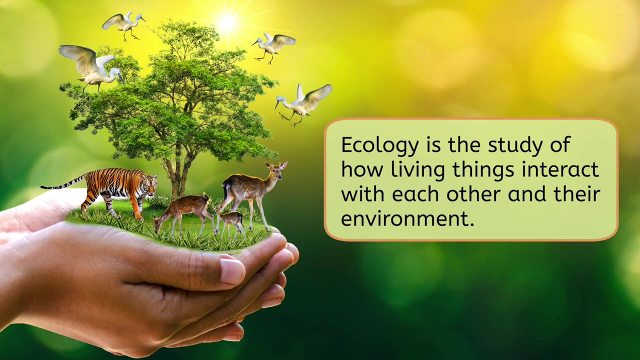 and differentiate between the various biomes that exist within it. Let's get into it. Ecology is the study of how living things interact with each other and their environment. This field of biology is really cool because it takes a lot of what we've been learning. 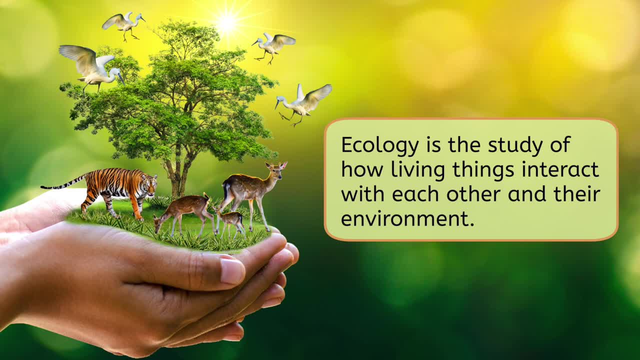 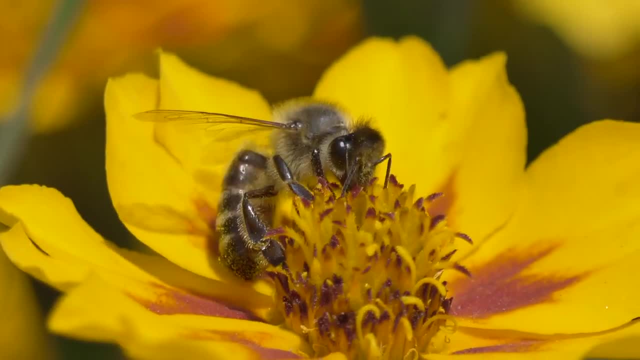 such as cellular processes, genetics and biodiversity, and allows us to examine the relationship between them. By studying this field of science, we gain a deeper understanding of how all living things are connected, which in turn allows us to make more informed decisions about. 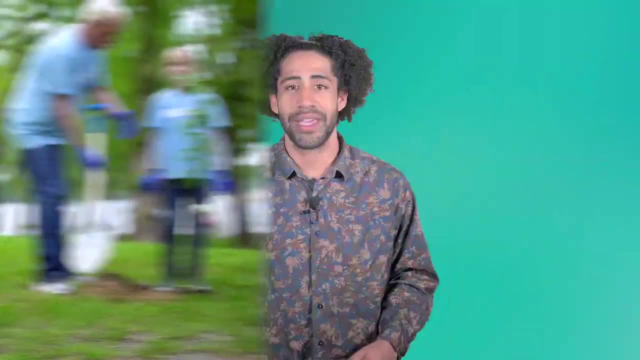 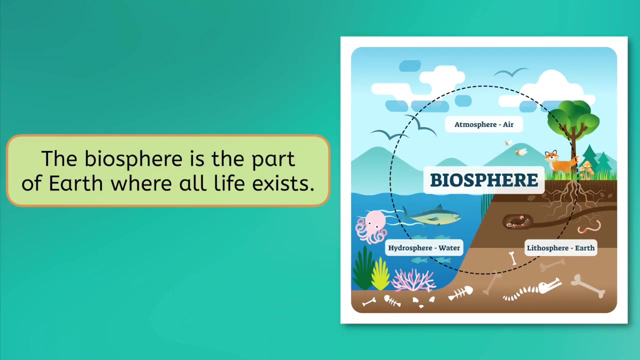 how we choose to interact with the world. To begin, let's talk about what makes our planet so special: the biosphere. This is the part of the Earth where all life exists. You're sitting in it right now. It includes the lithosphere, or land beneath our feet. 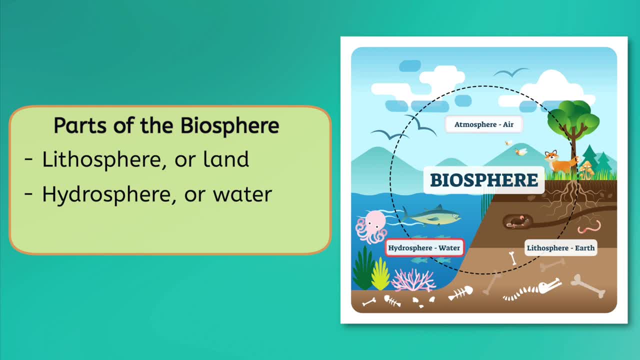 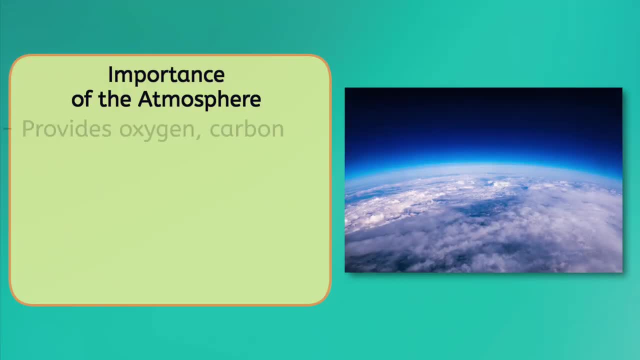 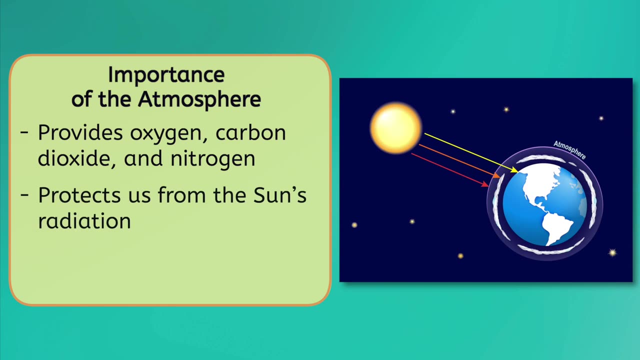 the hydrosphere, or water in our oceans and lakes, and the atmosphere, which is made up of the air we breathe. The atmosphere is important not only because it provides life-giving resources like oxygen, carbon dioxide and nitrogen, but it also protects us from the sun's radiation. 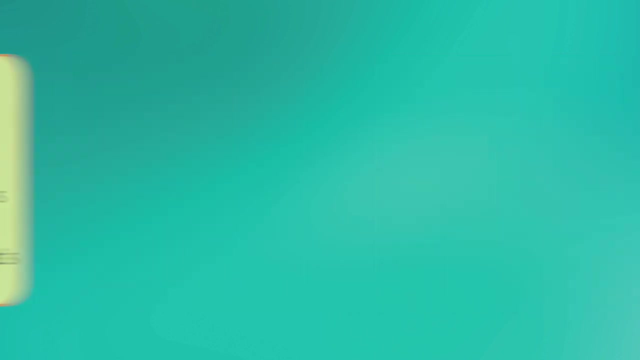 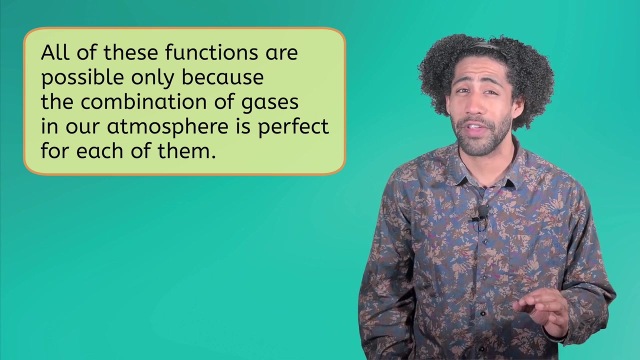 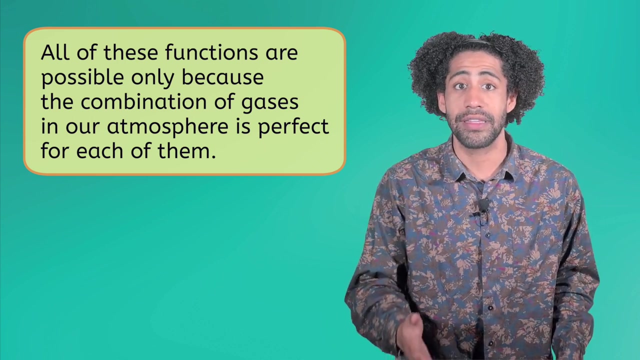 and helps regulate the planet's temperature. All of these functions are possible only because the combination of gases in our atmosphere is perfect for each of them. If the amount of oxygen, carbon dioxide or nitrogen in the atmosphere was different, life here wouldn't be possible. 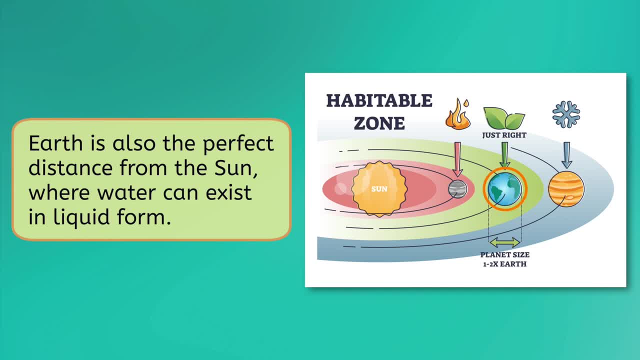 Another reason Earth is special is because it's the perfect distance from the sun where water can exist in liquid form. If it was significantly closer, Earth would be too hot for life, boiling the precious water away. If it was significantly farther, it would be too cold. 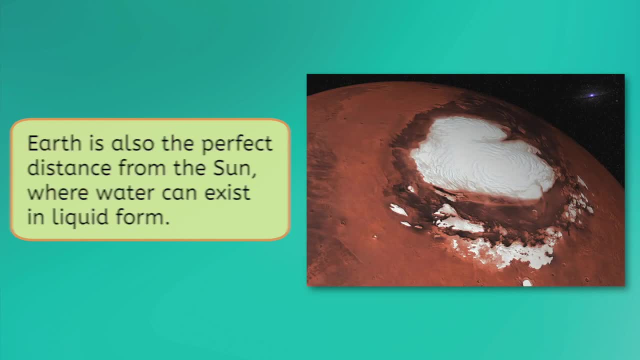 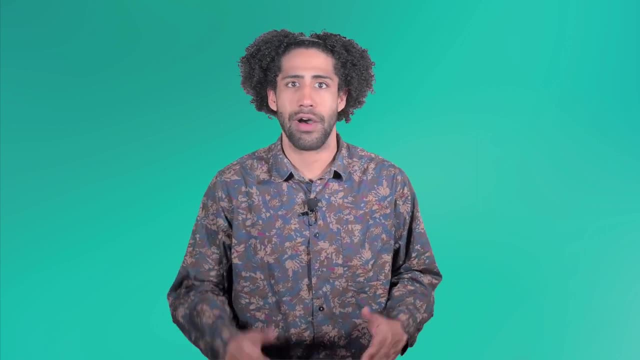 like Mars, where water only exists as ice. However, just because conditions in general are perfect for life doesn't mean that the biosphere is all exactly the same. Earth is constantly revolving around the sun and the atmosphere is constantly revolving around it. 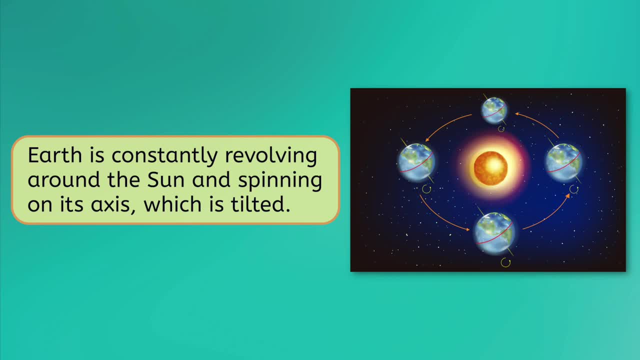 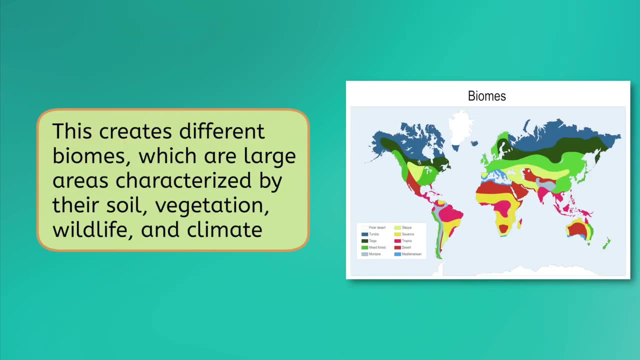 Earth is constantly revolving around the sun and spinning on its axis, which is tilted, so different parts of the planet are exposed to varying amounts of sunlight. This creates variations within the biosphere, called biomes, which are large areas characterized by their soil, vegetation, wildlife, and climate or weather. 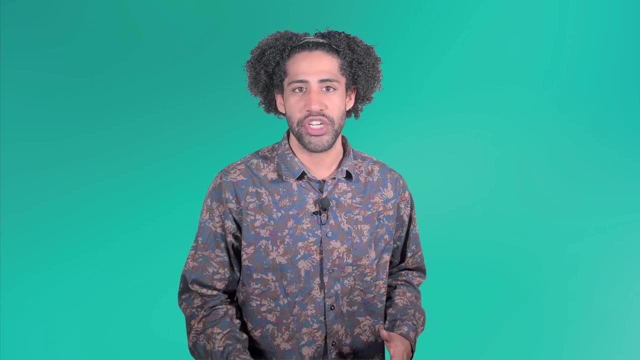 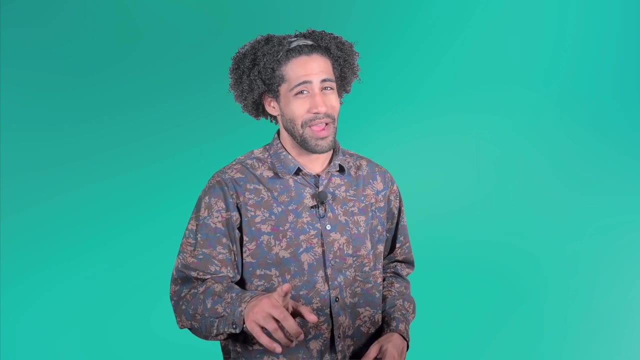 Studying biomes gives a larger perspective and appreciation of the diversity of life on Earth. Are you ready to explore these biomes with me Before we start? what kind of biome do you think exists on the planet? Write your thoughts in your guided notes. 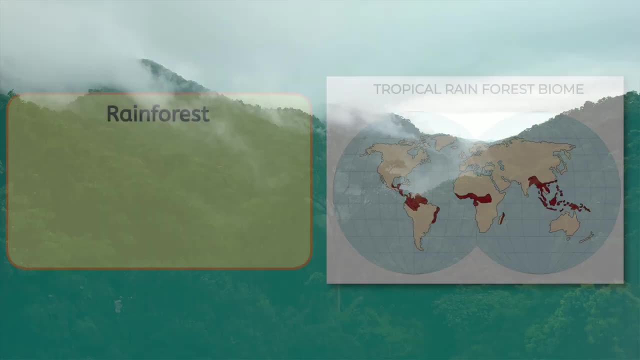 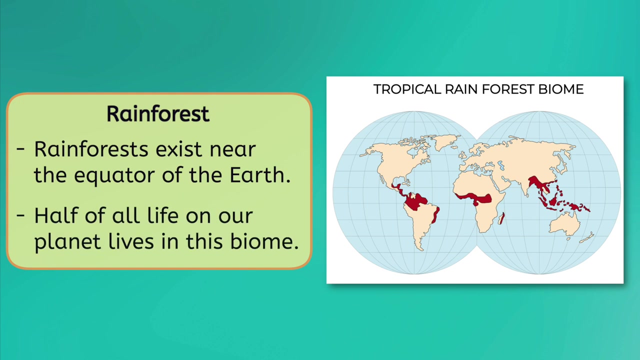 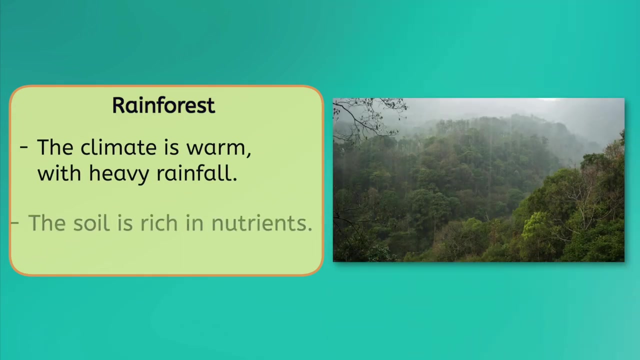 The first biome we'll be discussing is the rainforest. Rainforests exist near the equator of the Earth and half of all life on our planet exists in this biome. The climate is perfect for life: it's warm, with heavy rainfall, and the soil is rich in. 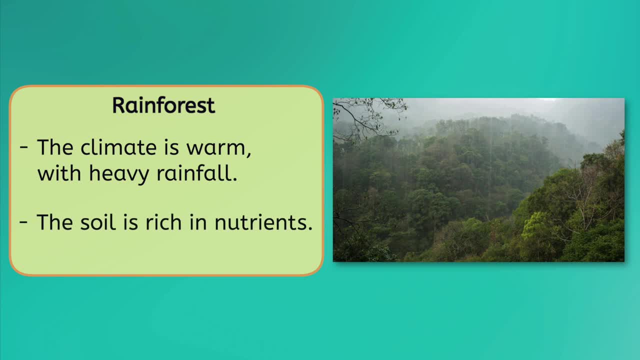 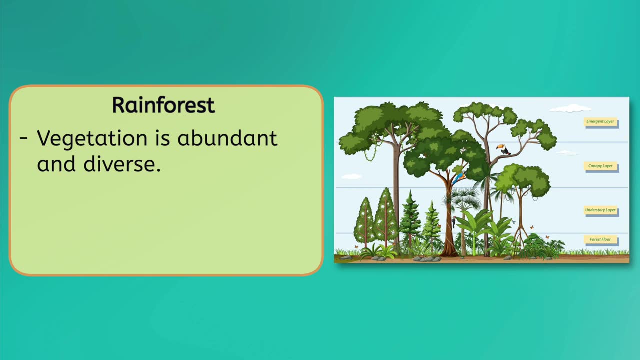 nutrients and organic matter, making it a perfect environment for life. The vegetation in a rainforest is abundant, with tall trees, lush ferns and a variety of climbing vines and shrubs. This allows for a complex network of life that includes many species. 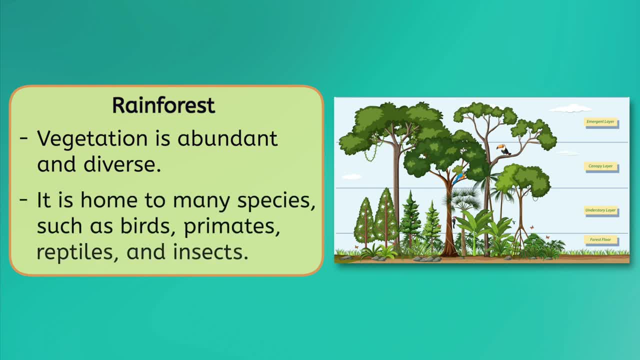 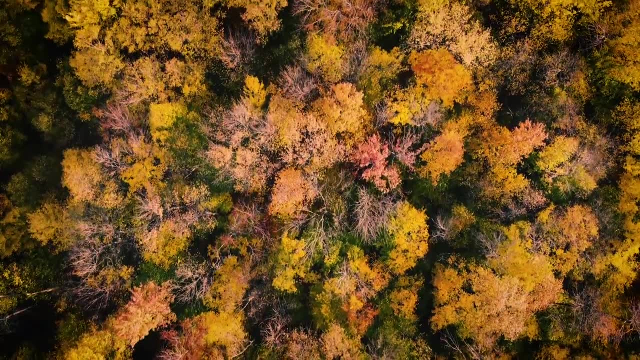 such as birds, primates, reptiles and insects. A temperate forest is a type of forest found in areas with moderate climates, typically in regions with four distinct seasons. If you live in an area with seasons, you should be aware of the fact that there are many different. 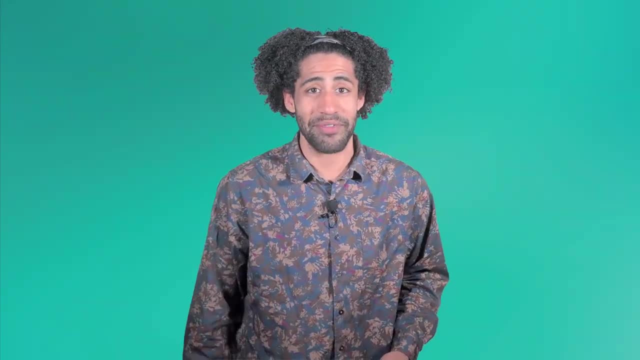 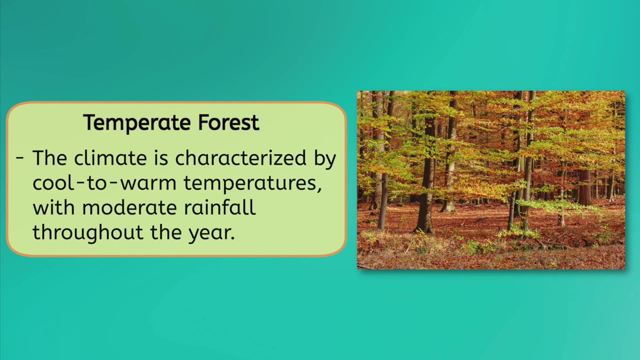 climates in the world. There are many different types of climates and there are many different seasons. You probably have these near you. The climate is characterized by cool to warm temperatures, with moderate rainfall throughout the year. The soil in a temperate forest is fertile. 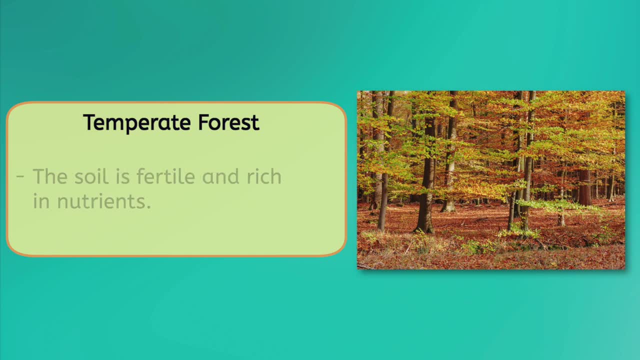 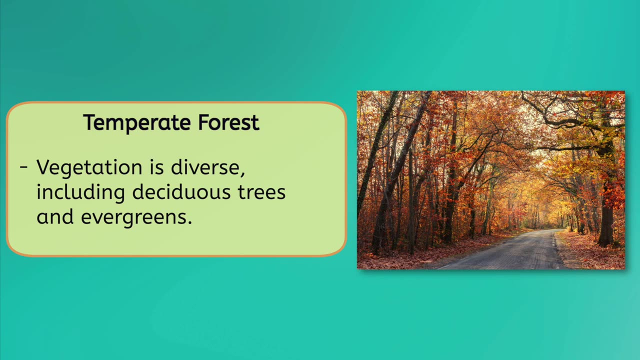 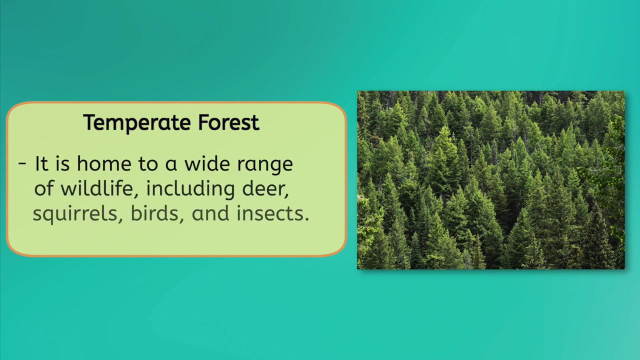 and rich in nutrients, supporting a variety of vegetation. This includes deciduous trees such as oak, maple and birch, which shed their leaves annually, as well as evergreens like pines and firs. The dense canopy created by the trees provides a habitat for a wide range of wildlife. 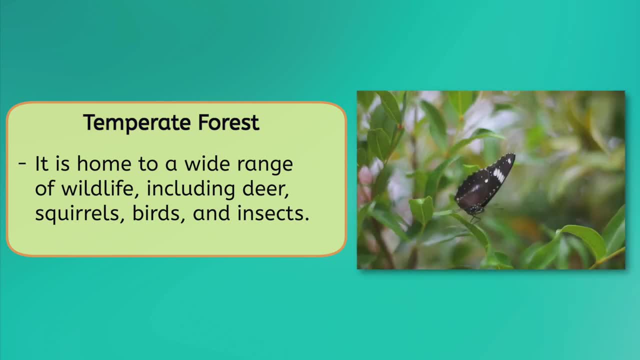 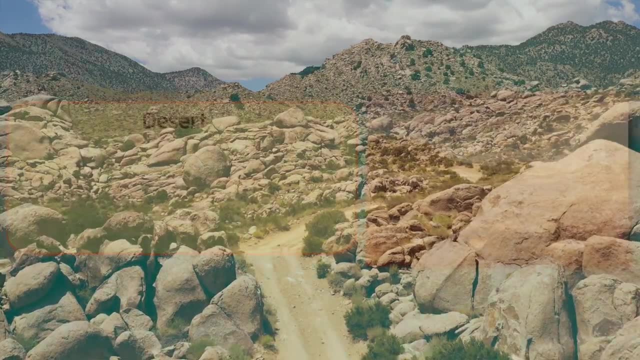 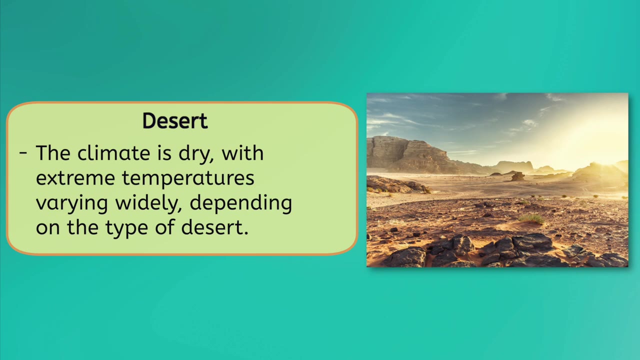 This includes deer, squirrels, birds and insects. A desert is a harsh environment with very little rainfall and extreme temperatures. It's characterized by a climate that is dry, with temperatures varying widely depending on the type of desert. Many deserts are very hot. 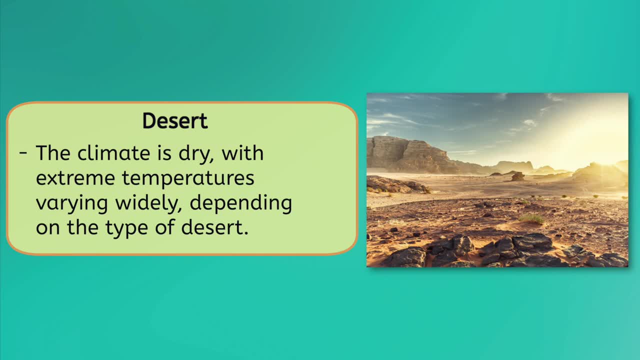 during the day and cold at night, while some, like polar deserts, are frozen solid year-round. The soil in a desert is typically rocky and sandy, with limited humidity, nutrients and water available for plant growth. As a result, vegetation in a desert is scarce. 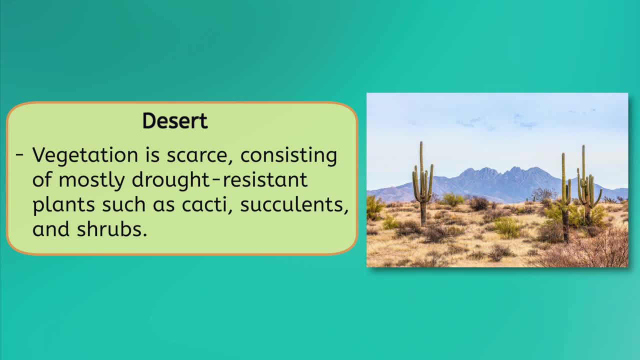 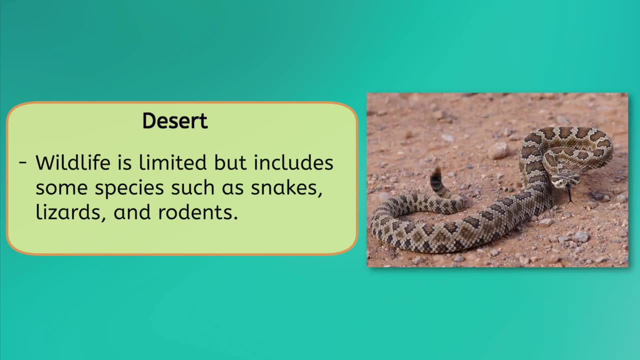 and consists primarily of drought-resistant plants such as cacti, succulents and shrubs. Despite the harsh conditions, some species of wildlife, such as snakes, lizards and rodents, have adapted to the desert environment and are able to survive in this ecosystem. 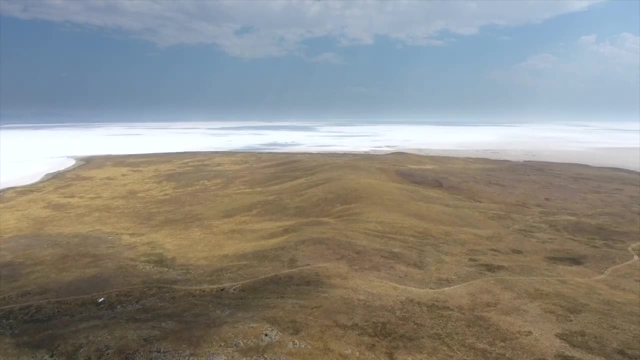 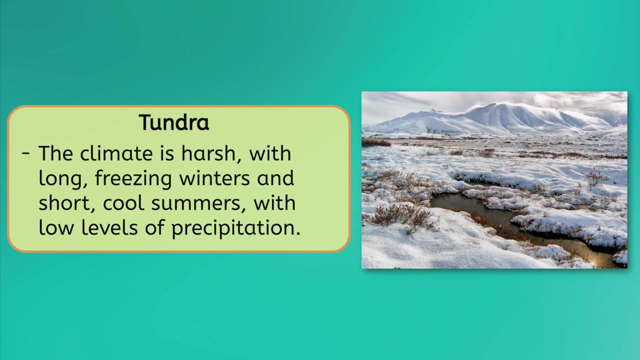 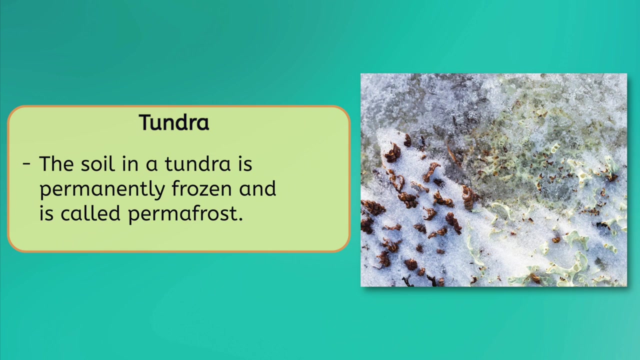 A tundra is a treeless and barren landscape found near the North and South Poles. Its characteristics include a climate that is harsh, with long freezing winters and short cool summers with low levels of precipitation. The soil in a tundra is permanently frozen. 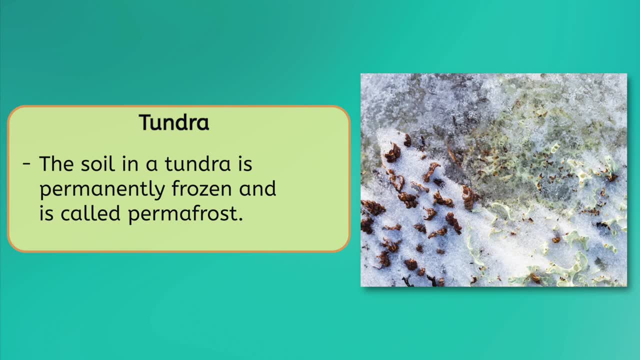 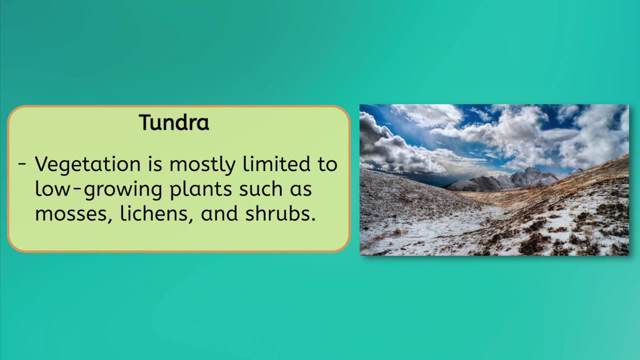 known as permafrost, making it difficult for plants to take root and grow. Vegetation in a tundra is limited to low-growing plants such as mosses, lichens and shrubs, as well as a few hardy flowers that bloom briefly in the summer Despite the harsh conditions. 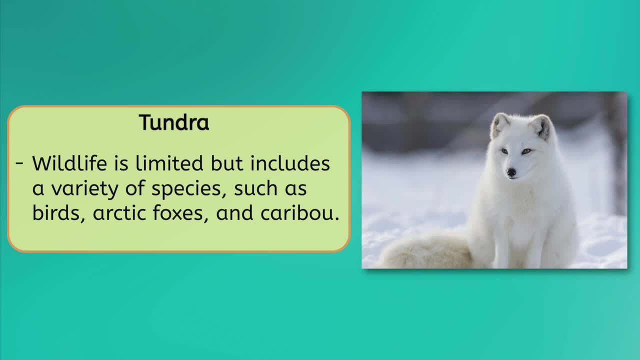 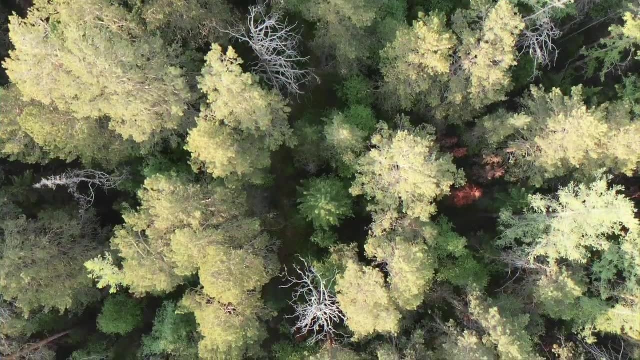 a variety of wildlife, such as birds, arctic foxes and caribou, have adapted to the tundra and are able to survive in this unique environment. A boreal forest, also known as a taiga, is a type of forest typically found in the northern hemisphere. As far as its characteristics, 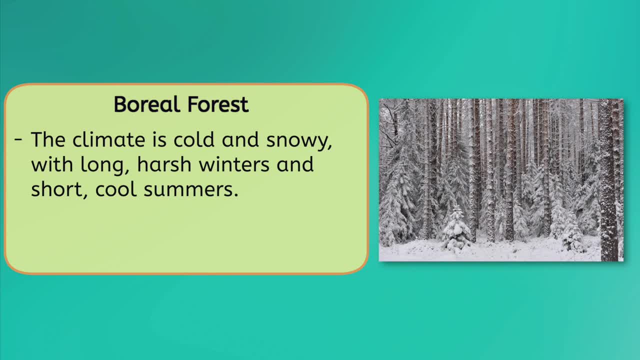 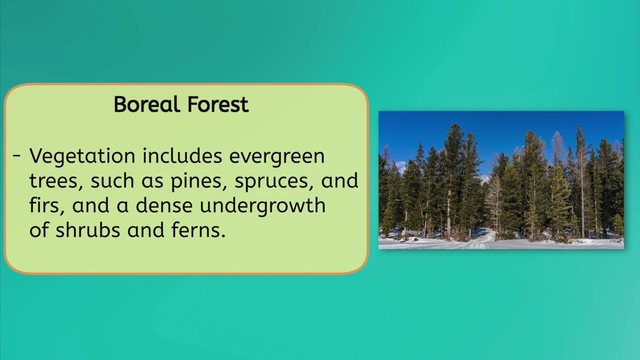 go. the climate is cold and snowy, with long harsh winters and short cool summers. The soil in a boreal forest is typically nutrient-rich and well-drained, supporting a variety of vegetation. This includes evergreen trees such as pines, spruces and firs. 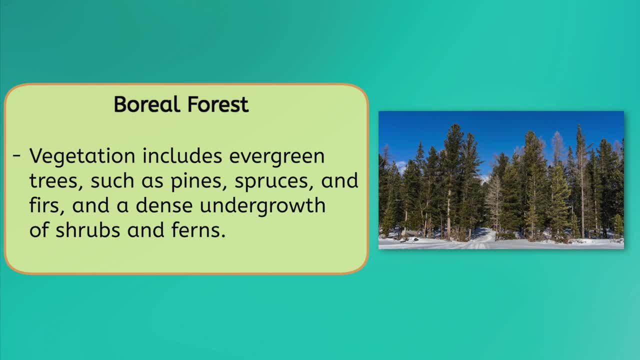 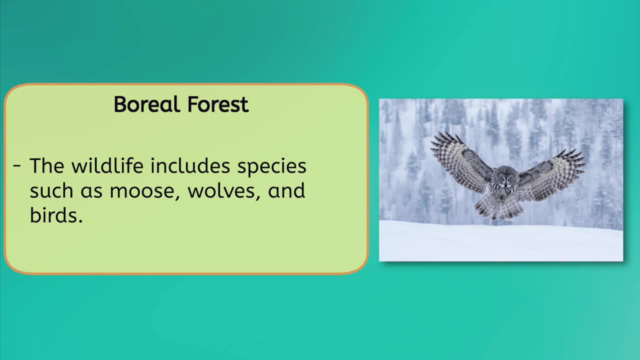 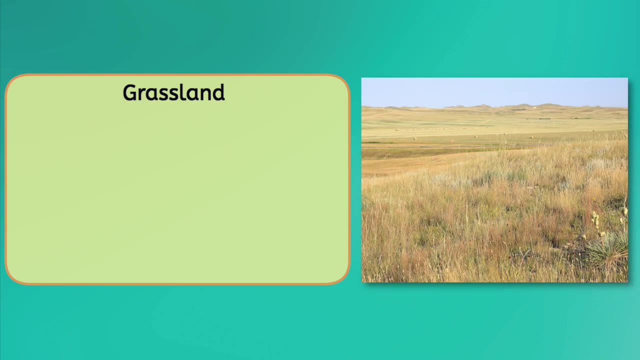 and a dense undergrowth of shrubs and ferns. Despite the harsh conditions, a variety of wildlife, such as moose, wolves and birds have adapted to the boreal forest and are able to survive and thrive in this unique environment. A grassland is a vast and rolling landscape. 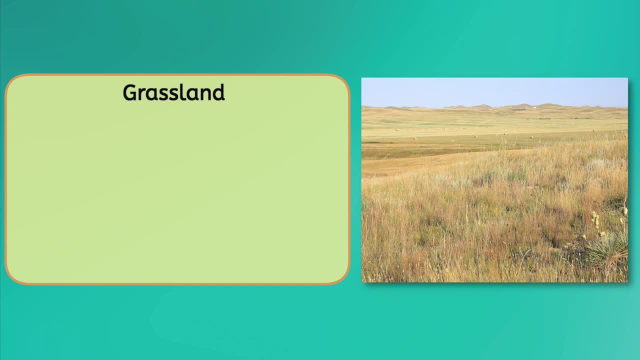 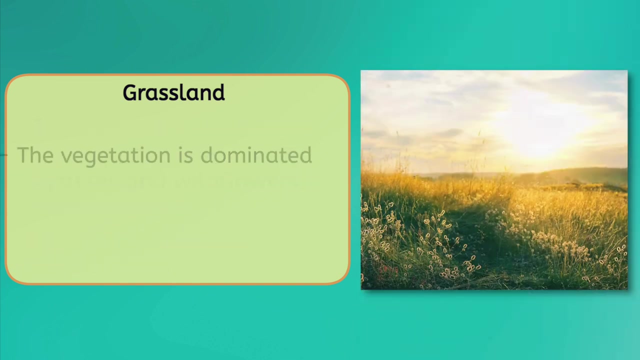 dominated by grasses and other low-growing plants. The climate is characterized by moderate temperatures and moderate to low levels of precipitation, with long hot summers and short cool winters. The soil in a grassland is fertile and well-drained, and the vegetation is dominated.